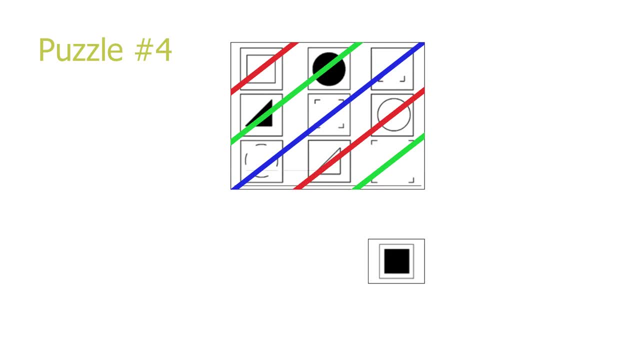 where there is a repetition of black shapes, The answer is a square and it's black. 3 is the correct solution. Puzzle 5.. Another diagonal puzzle: On the top right to bottom left diagonals, we have a repetition of pictures. 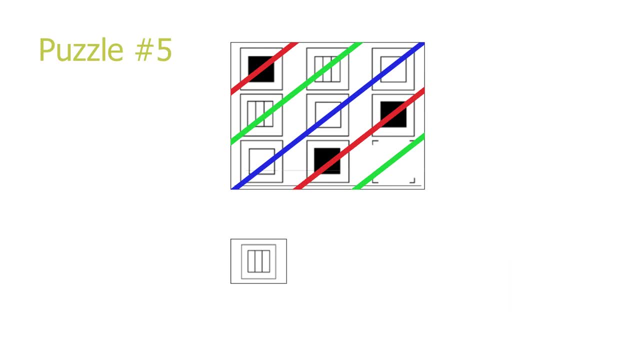 Our answer is in the green diagonal, where we have a repetition of squares with two vertical lines inside of them. 1 is the correct answer, Puzzle 6.. To solve this puzzle, let's start by looking at the first row, Going from picture 1 to picture 2, we see a 90 degree clockwise rotation and going 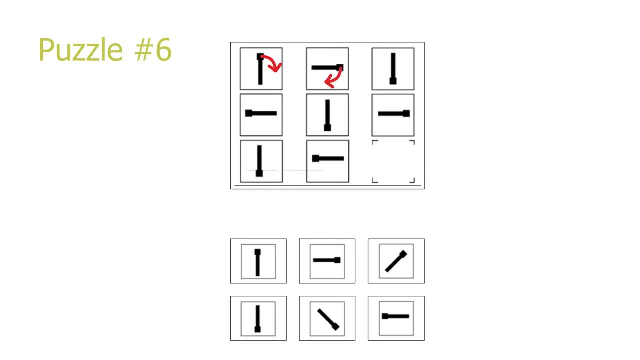 from picture 2 to picture 3, we also see a 90 degree clockwise rotation. Now let's look at the second row. We first see a 90 degree counterclockwise rotation and then another 90 degree counterclockwise. 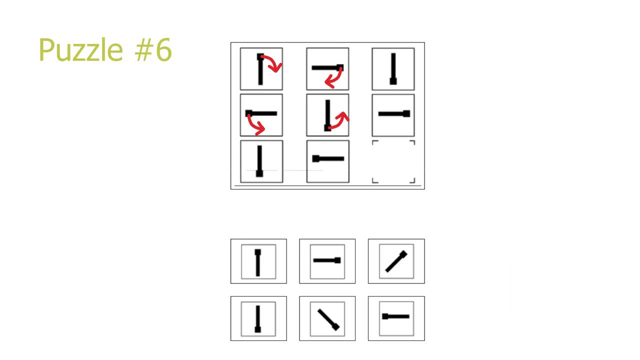 rotation. Therefore we know that the first rotation going from picture 1 to picture 2 is also the same rotation going from picture 2 to picture 3.. Looking at the last row, we first have a 90 degree clockwise rotation, so we should. 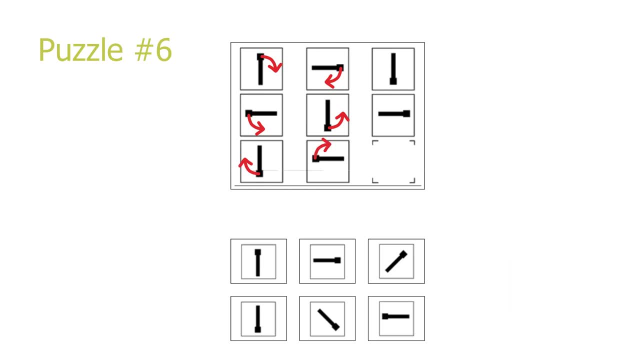 have another 90 degree clockwise rotation going from picture 2 to picture 3. This leads to a picture pointing upwards. Answer 1 is the correct solution. Puzzle 7. Here we have the exact same puzzle as the previous one, just with arrows instead. 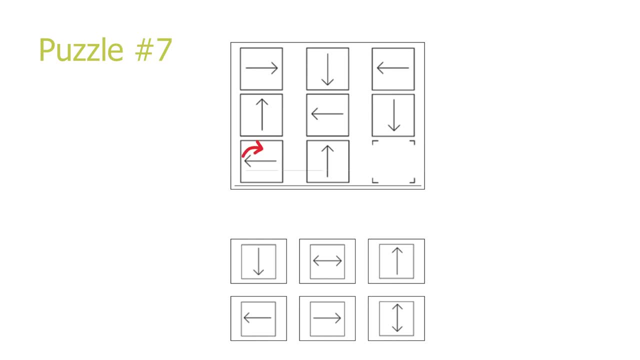 Going by the last row. we first have a 90 degree clockwise rotation and therefore we should have another 90 degree clockwise rotation going from picture 2 to picture 3.. This leads to an arrow pointing upwards. Answer 5 is the correct solution. 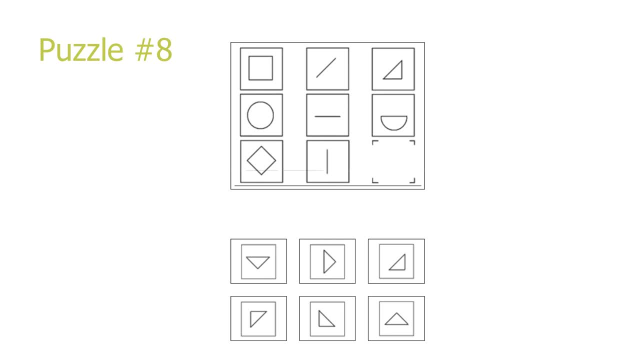 Puzzle 8.. This is a row puzzle To give you a visualization of how we go from the first and second picture in a row to the third picture. let's use the first row as an example. First we take picture 1, then we add picture 2 on top of it. 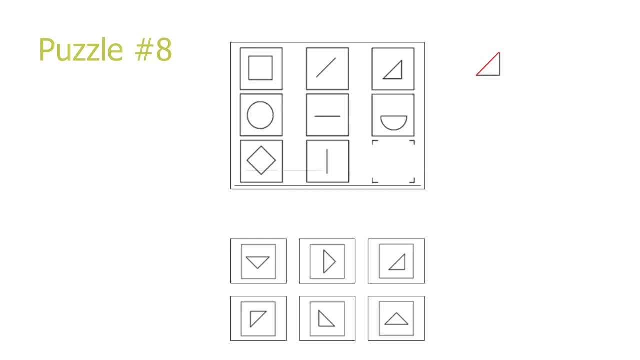 We can see that picture 2 cuts picture 1 in half and if we remove one of these halves we get a triangle shape. And if I now turn picture 2 black, we can see that it's identical to the third picture in the first row. 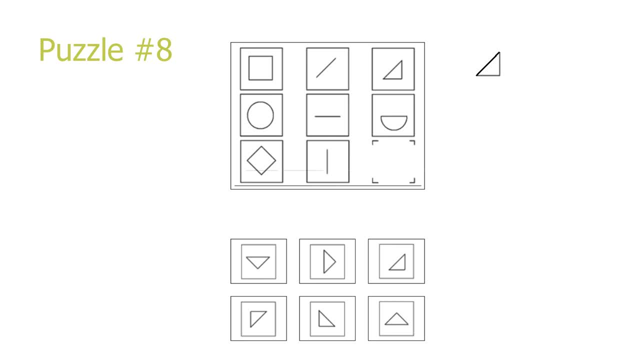 Doing the same with the last row. we have this diamond shape and a vertical line. The vertical line cuts the diamond shape in half and leaves a triangle pointing towards the right. Answer. 2 is the correct solution. Puzzle 9.. This is a row and column puzzle. 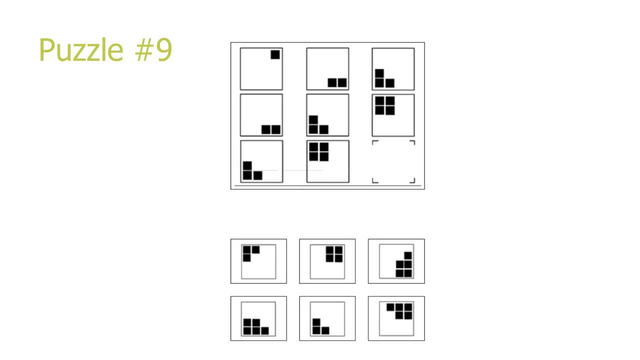 Moving to the right in a row or moving downwards in a column has the same effect. Both leads to a 90 degree clockwise rotation and an addition of one more square in a cluster of squares. Looking at the last row, we can take the second picture and rotate it 90 degrees clockwise. 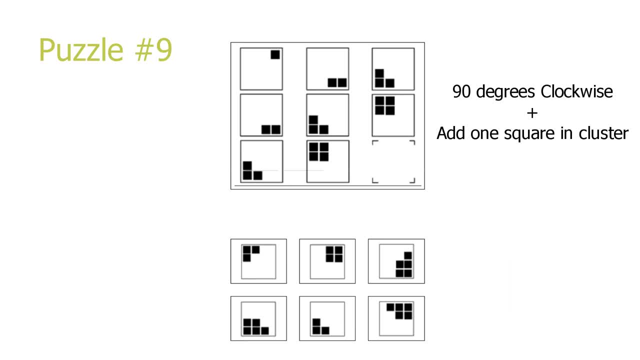 and add another square to get a 90 degree clockwise rotation. This leads to a picture with 5 black squares in the top right corner. Answer 6 is the correct solution. Puzzle 10.. This is very similar to the previous puzzle, just even easier. 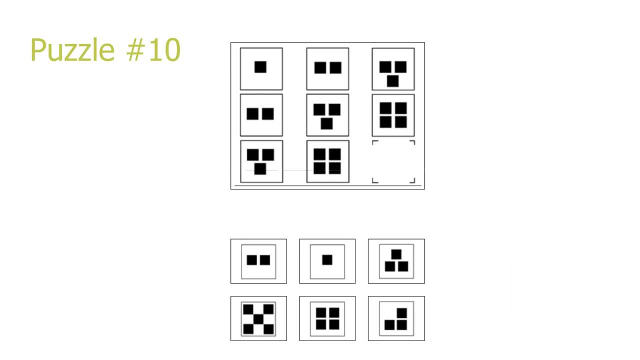 Moving to the right in a row or moving downwards in a column leads to both adding a new square. Going by the last row, we see that the second picture has 4 squares, and moving once to the right adds a new square, So our answer will have 5 squares. 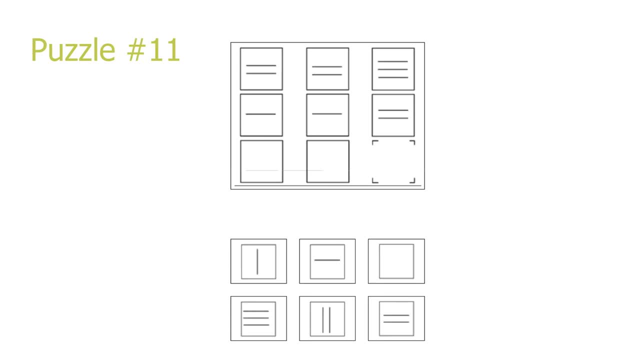 Answer 4 is the correct solution. Puzzle 11.. This is a column puzzle. Moving downwards in a column leads to one horizontal line being removed. Looking at the last column in the second picture we have two horizontal lines Moving down to our answer will remove one of these lines. 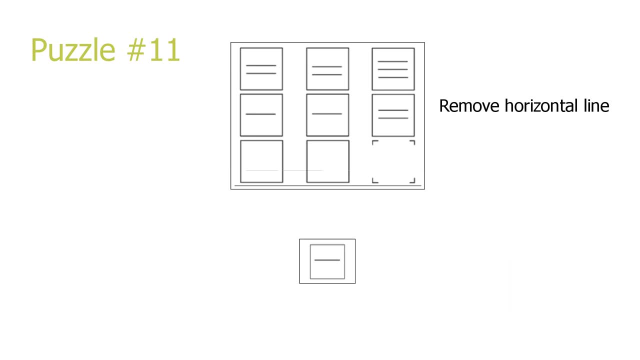 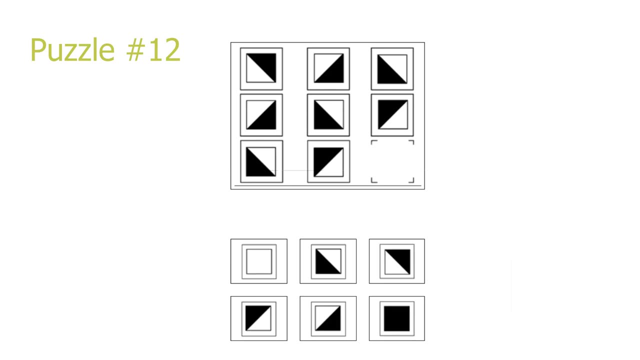 Therefore, our answer will be a single horizontal line. Answer 2 is the correct solution. Puzzle 12.. In this puzzle, moving downwards in a column and moving to the right in a row has the same effect. Both leads to a rotation of 90 degrees in clockwise direction. 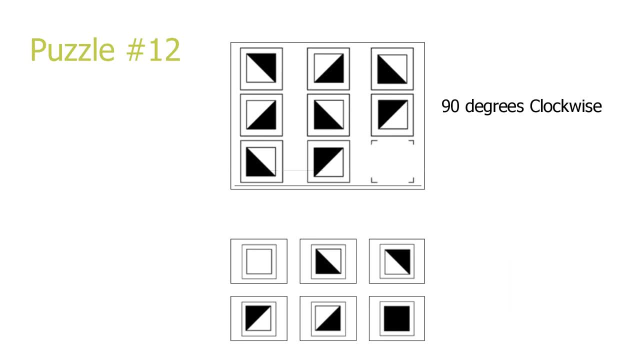 To solve the puzzle, let's look at the last row. The second picture is pointing towards the top left. Rotating it 90 degrees clockwise will lead to a picture pointing towards the top right. Answer 3 is the correct solution. Puzzle 13.. 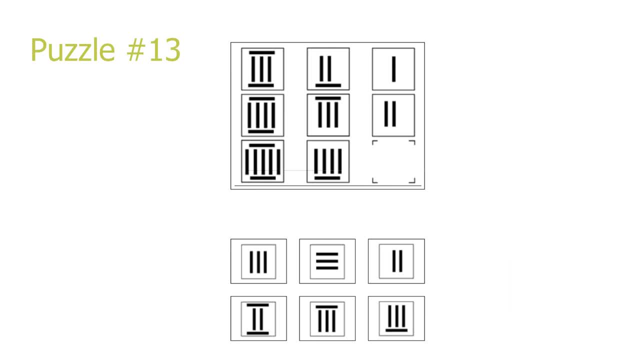 This is a row and column puzzle. We can either solve it by the columns or the rows. Moving down in a column leads to a new vertical line being added into the picture, Going by the last column. we see that in the second picture we have two vertical lines. 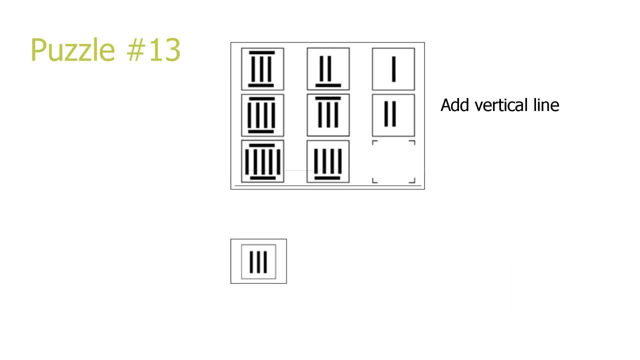 So, moving down to our answer, we just add a new vertical line and we get three vertical lines. Answer 1 is the correct solution. Puzzle 13. Puzzle 14.. I highly suggest solving this puzzle by looking at the columns. Looking at the first column, we can see how rotating the first picture 90 degrees leads. 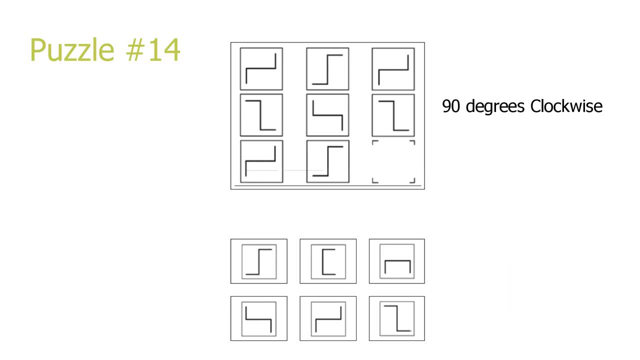 to the second picture, and rotating the second picture 90 degrees leads to the third picture. To solve the puzzle, let's do the same for the last column. We rotate the second picture in the last column by 90 degrees. This leads to 5 being the correct solution. 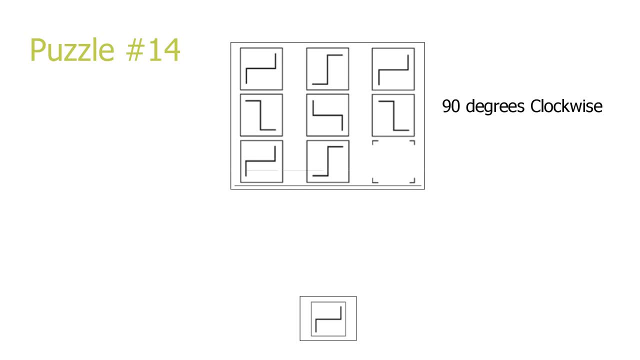 As a side note, if we look at the first picture in the column, it's identical to its third picture, So to solve the puzzle, we could have just found the answer here. Answer 3 is the correct solution. Answer 4 is the correct solution. 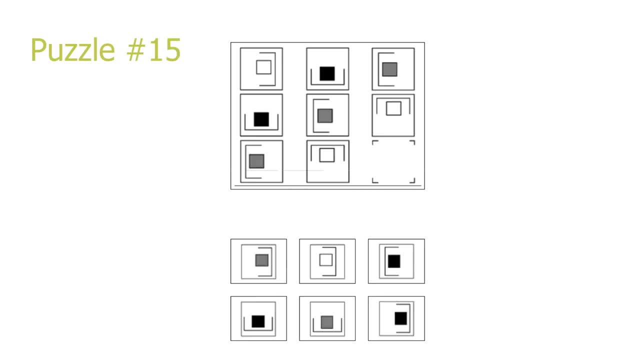 Answer 5 is the correct solution. Hence we got an answer which was identical to the first picture in the third column, Puzzle 15.. This is a combination of puzzles. First let's take a look at the top right to bottom left diagonals. 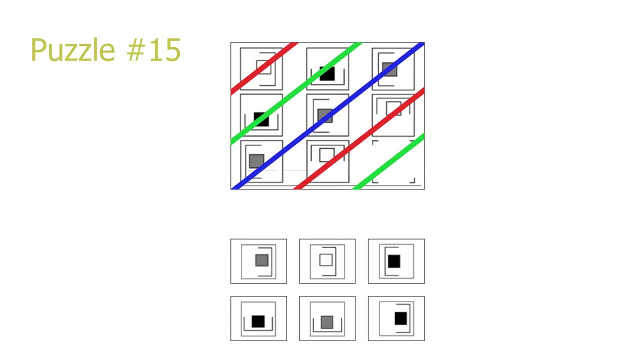 On these diagonals there is a repetition of the color inside of the squares. Our answer is in the green diagonal, which have a repetition of black squares. therefore, our answer will contain a black square. This leaves answer 3,, 4 or 6 as the correct answer. 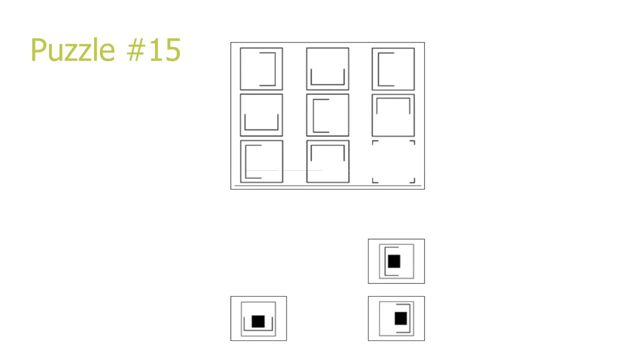 Secondly, if we only look at the rest of the shape in the pictures, we can see that it's 90 degrees clockwise. if we either move downwards in a column or to the right in a row, Going by the last row, we can rotate the second picture 90 degrees clockwise in order to get. 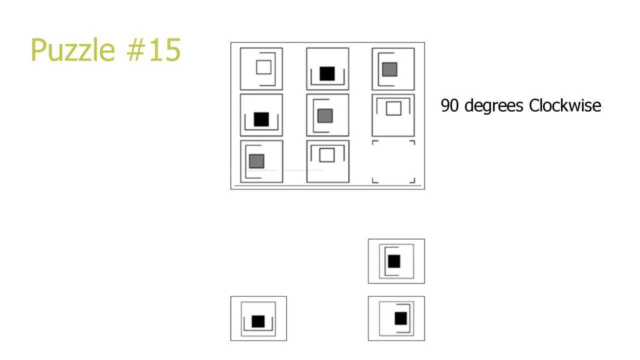 the shape in our answer. The second picture is pointing upwards and rotating it 90 degrees will make it point towards the right Answer. 6 is the correct solution. Puzzle 16.. This is a round column puzzle. This is a pretty hard puzzle to visualize. going from picture to picture. 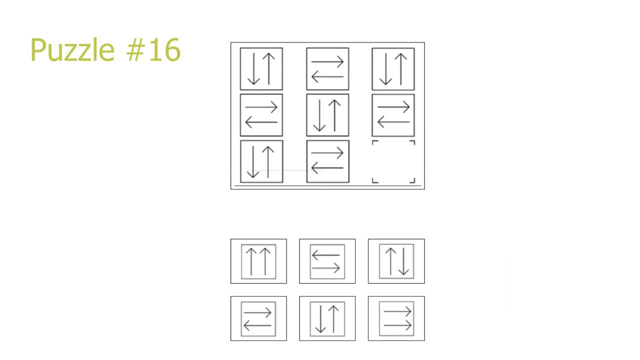 If you look at the first row, to go from the first picture to the second picture, we have to mirror the image across these axes. But yeah, knowing this mirroring is irrelevant because if we look at the first and the third row, they are identical. 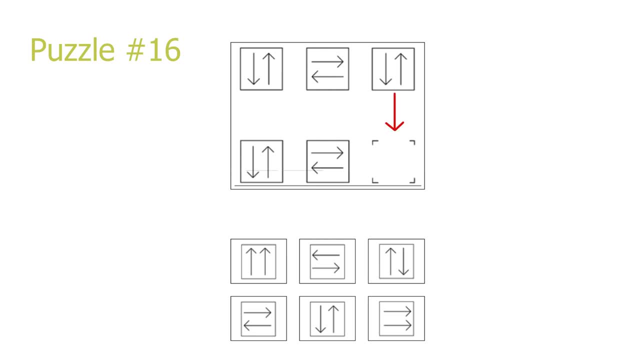 So the third picture in the third row will be identical to the third picture in the first row. Answer 5 is identical to picture 3.. Therefore, answer 5 is the correct solution. Puzzle 17.. This is a round column puzzle. The easiest way to solve it is by looking at the columns. 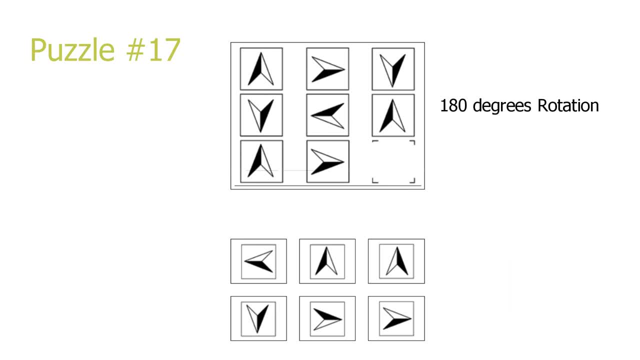 Moving down in a column, we just rotate the picture 180 degrees to create the next picture. For a short mental shortcut, notice that moving downwards twice in a column is the same as rotating the picture 360 degrees. A 360 degree rotation is a full rotation, so the first picture in the column will be identical. 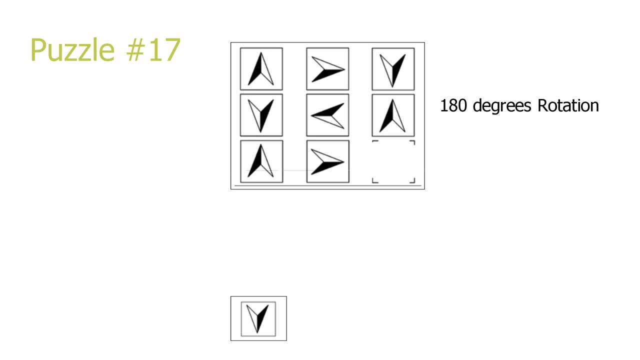 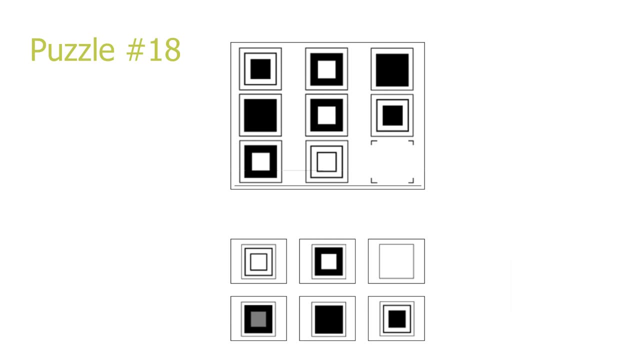 to the third picture, Our answer will be identical to the first picture in the third column. Answer 4 is the correct solution, Puzzle 18.. This is an addition puzzle with cancellation. To produce the third picture in the row or column, we just add the first and the second. 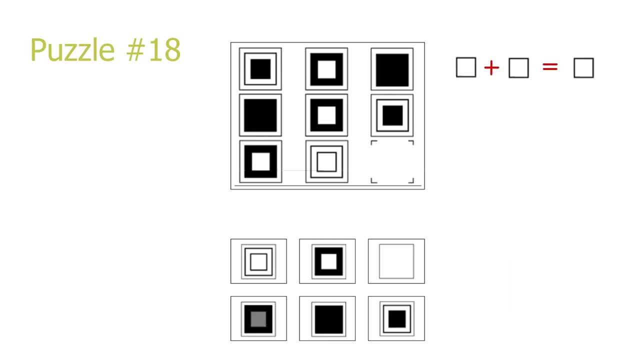 picture. The rules are as following: If we add the two white areas, Then we get a white column, Then we get a white area in the third picture. If we add one black area and one white area, then we get a black area in the third picture. 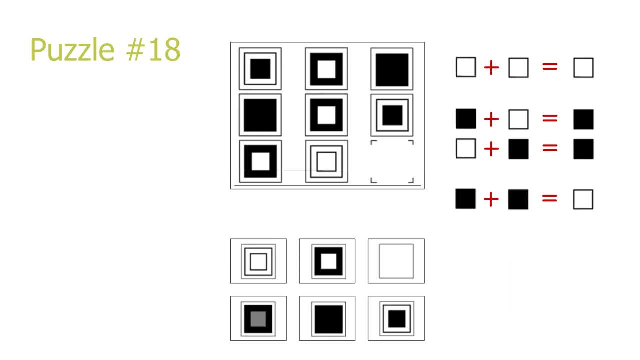 And finally, if we add two black areas, then we get a white area in the third picture. There are more puzzles like this in the test. so whenever I say addition puzzle with cancellation, these are the rules that the puzzle will follow. In this puzzle we have two areas which obey these rules. 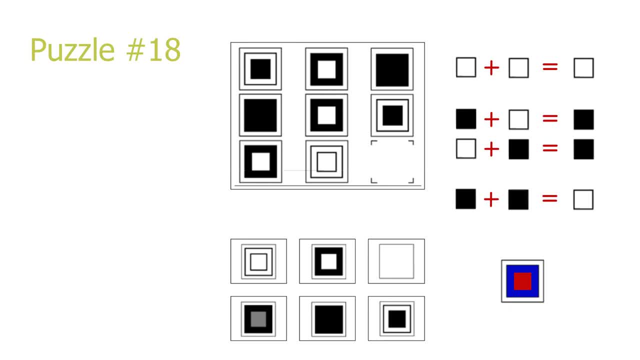 We have the outer area, which are marked in blue, and the inner area, which are marked in red. Looking at the last row, the first picture has a black outer area and a white inner area. in the second picture This leads to our answer having a black outer area and a white inner area. 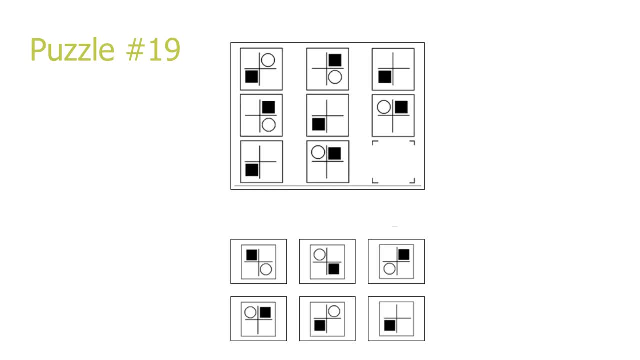 2 is the correct answer. Puzzle 19. This is a puzzle where moving downwards in a column and moving to the right in a row has the same effect. Let's start by focusing only on the black squares. The black squares always moves two positions in clockwise direction when moving to the. 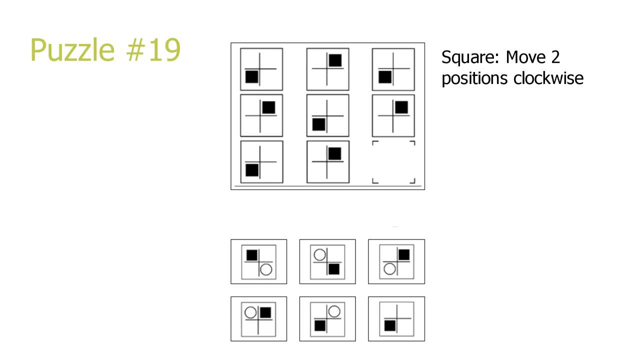 right in a row To find out in what corner our answer will have a black square. let's look at the last row. In the second picture we have a black square in the top right corner. Moving it in two positions in clockwise direction leads to a black square in the bottom left. 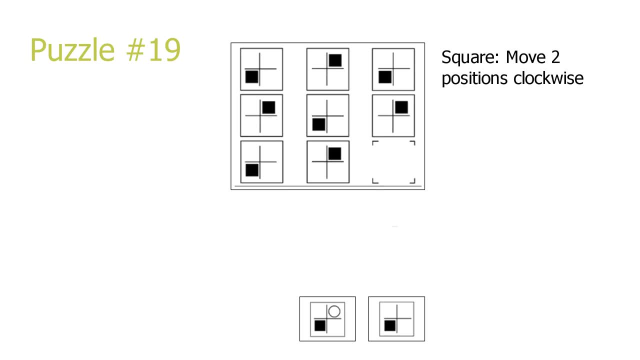 corner. Therefore, our answer will have a square in the bottom left corner. This leaves either answer 5 or 6 as the correct answer For the circles. we see that moving to the right in a row leads to the circle moving in one position in clockwise direction. 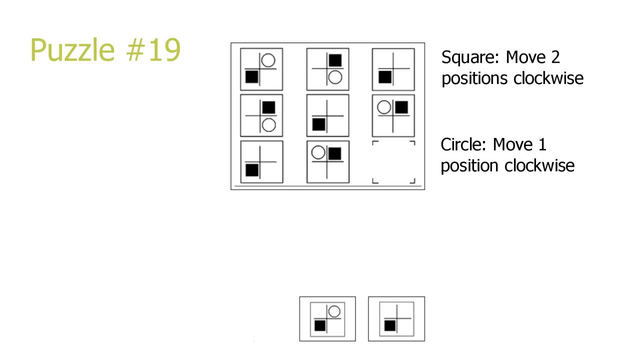 Also, if the circle and the square is in the same position, then the square will show instead of the circle. To solve the puzzle, let's look at the last row. We see that the second picture in the last row has a circle in the top left corner. 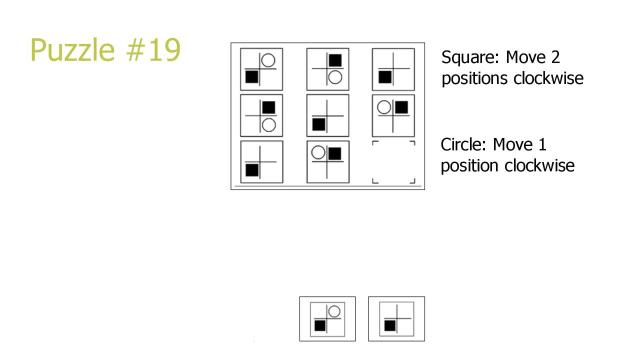 Moving this circle once in clockwise direction leads to our answer having a circle in the top right corner. Our answer will have a circle in the top right corner and a square in the bottom left corner. 5 is the correct solution. Puzzle number 20.. 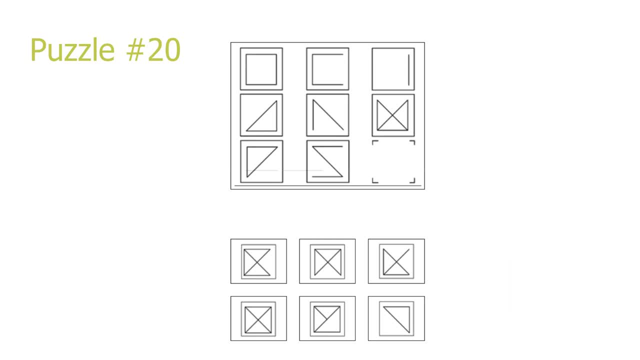 This is an addition puzzle with cancellation. The puzzle could either be solved in the rows or the columns. To solve the puzzle, let's look at the last column. The first picture in the third column is just a vertical line on the right side. The second picture also has this vertical line on the right side, so they cancel out. 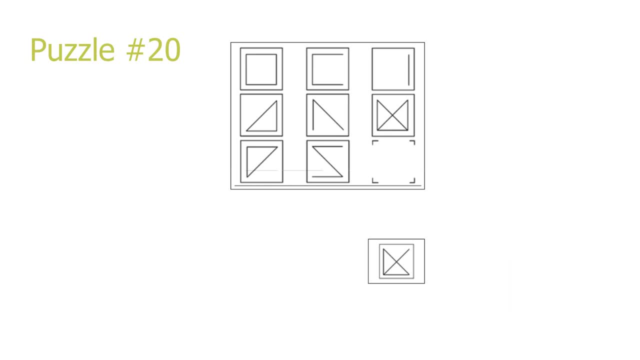 Therefore, our answer will be identical to the second picture in the third column with the vertical line on the right side removed. This leads to a picture identical to answer 3.. Answer 3 is the correct solution. Puzzle 21.. This is another addition puzzle with cancellation. 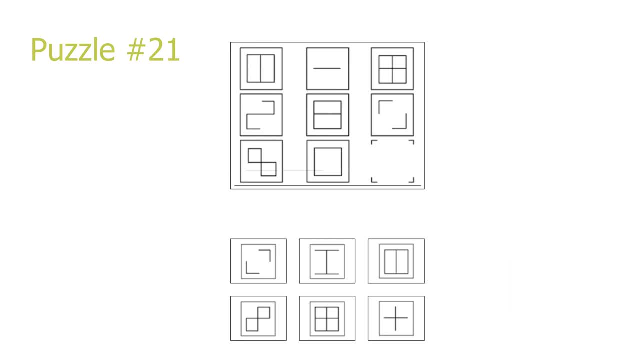 To solve the puzzle, let's look at the last row. The first picture is two small squares, one in the top left corner and one in the bottom right corner. The second picture is a big square. Solving the first and the second picture leads to a picture with two small squares. 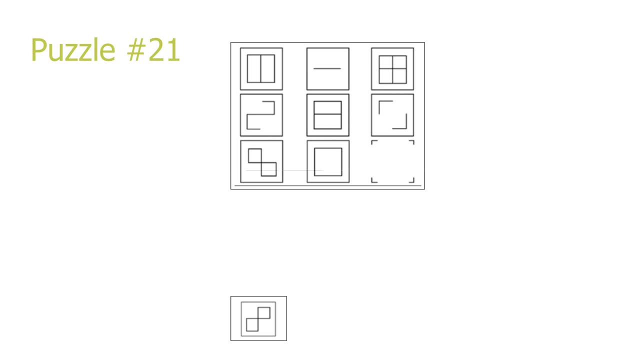 one in the top right corner and one in the bottom left corner. Answer 4 matches this description. Four is the correct solution. Puzzle 22. This is a puzzle where moving to the right in a row or moving downwards in a column has the same effect. 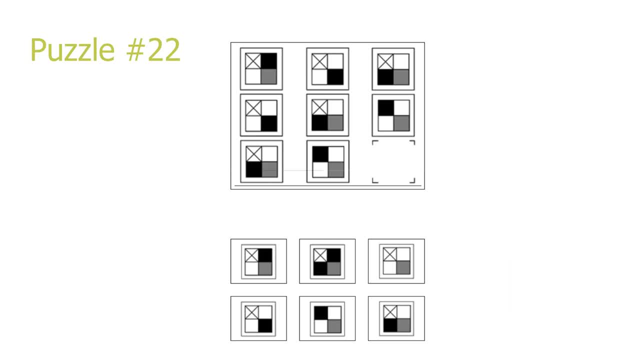 In this puzzle we have a square which is divided into four smaller squares. In the top left corner of every picture, we have an X shape, and in the bottom right corner of every picture we have a grey square. We also have this black square which moves in one position in the right. 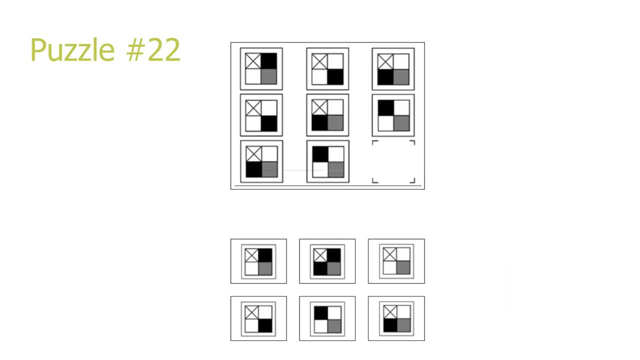 Puzzle 23.. Another puzzle where we have the same effect: moving to the right in a row or moving downwards in a column. To solve the puzzle, let's look at the last row. The second picture has a black square in the top left corner. 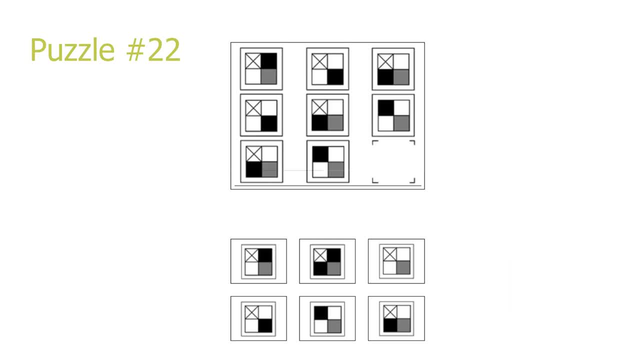 Moving it in one position in a clockwise direction leads to there being a black square in the top right corner in our answer And of course, we will have a grey square in the bottom right corner and an X in the top left corner. Answer 1 matches this description, so one is the correct solution. 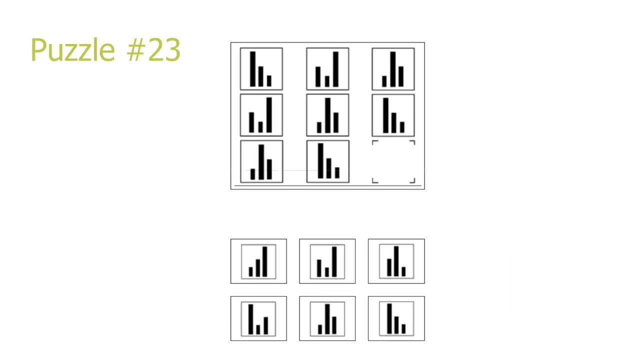 Puzzle 23.. Another puzzle where we have the same effect: moving to the right in a row or moving downwards in a column. Moving to the right in a row leads to other lines being moved in one position towards the left, while the leftmost line is moved to the rightmost position. 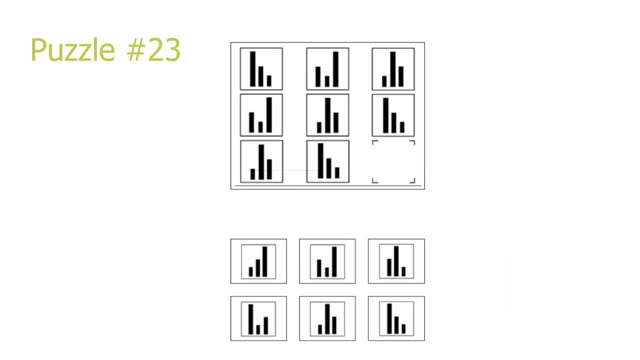 To solve the puzzle, let's look at the last row In the second picture. in the last row we have the biggest line in the leftmost position, so we know that our answer will have the biggest line in the rightmost position. Also, moving the other lines in one position towards the left leads to our answer having 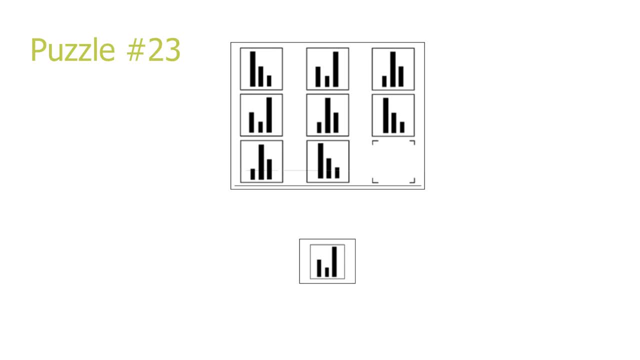 the second largest line on the left, the smallest line in the middle and the biggest line on the right. Answer 2 is the correct solution. Puzzle 24.. This is an addition puzzle with cancellation. The easiest way to solve the puzzle is by looking at the last column. 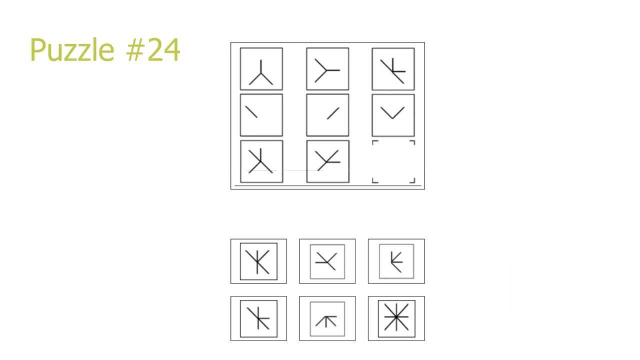 The first and second picture in the last column has a single line in common which reaches from the middle of the picture to the top left corner. After this line cancels out, they have four lines left. One line is pointing upwards, one is pointing towards the top right corner, one is pointing 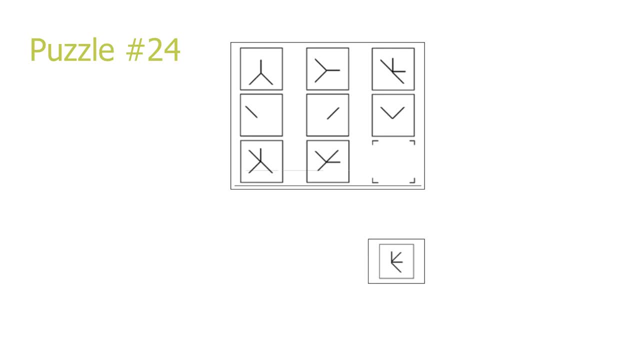 towards the right and the last line is pointing towards the bottom right corner. This leads to answer 3 being the correct solution. Puzzle 25.. This is a row puzzle, So all the pictures in the first column are identical. therefore, we have to base ourselves. 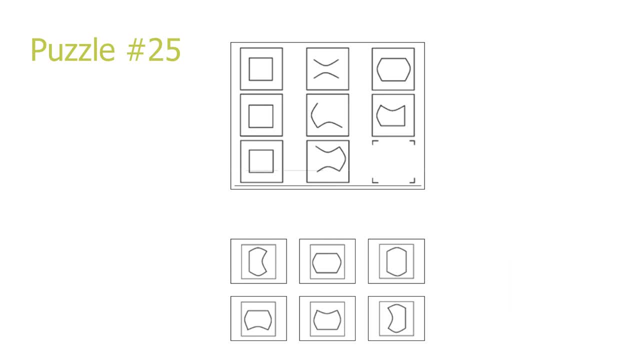 only on the second column to get the third column. Looking at the second column, we see that the first and second picture have this inward curve shape on the bottom in common. This will obviously lead to the same change in the third picture in row 1 and row 2.. 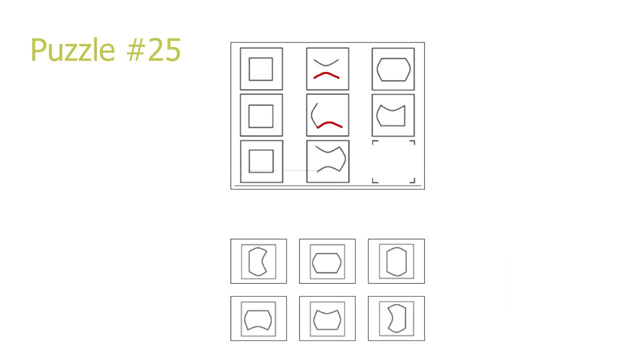 Looking at the third column, what does the first and second picture have in common? They have this outward curve on the left in common. Just as a short note, they also have this straight line on the bottom in common. but we can assume that a straight line is an unaffected line, because our base picture in the first 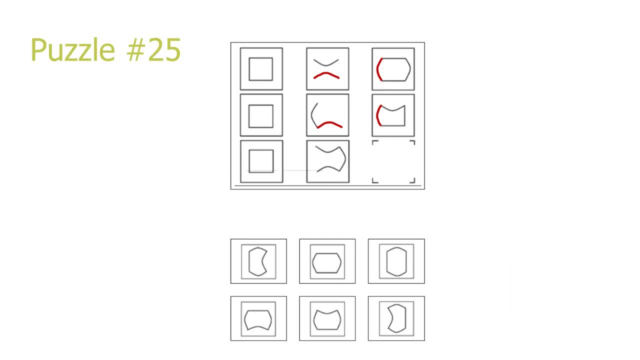 column is just a regular square, So an inward curve shape on the bottom in the second picture leads to an outward curve shape on the left in the third picture. Looking at the first row, we still have this inward curve on the top in the second picture. 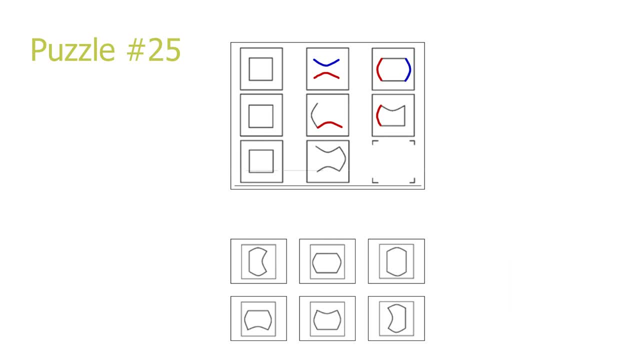 This of course corresponds to an outward curve shape on the right in the third picture. For the second row we have an outwards curve in the second picture. This corresponds to an inwards curve on the top in the third picture, Puzzle 26.. 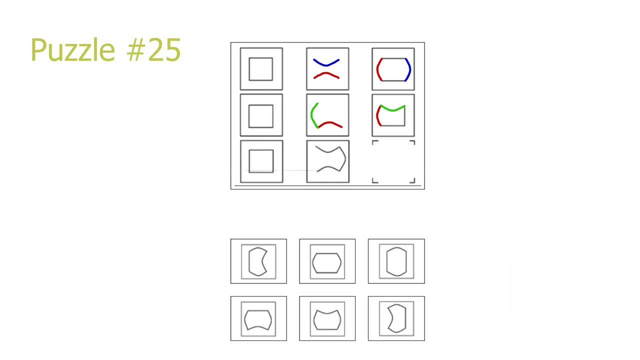 Notice that the effect on the third picture in a row always happens 90 degrees in a clockwise direction compared to where the change is described in the second picture. With this information I can see a clear transition to go from the second picture to the third picture in any given row. 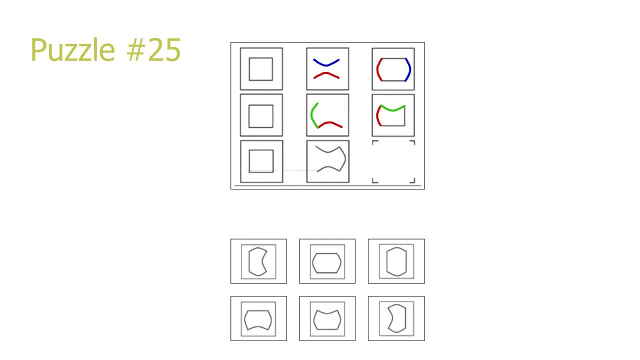 For you to see the same as I see in my head. let's use the first row as an example. We take the second picture in row 1, we rotate it 90 degrees clockwise. we invert the curvature so that inwards becomes outwards and outwards becomes inwards. we add the first picture. 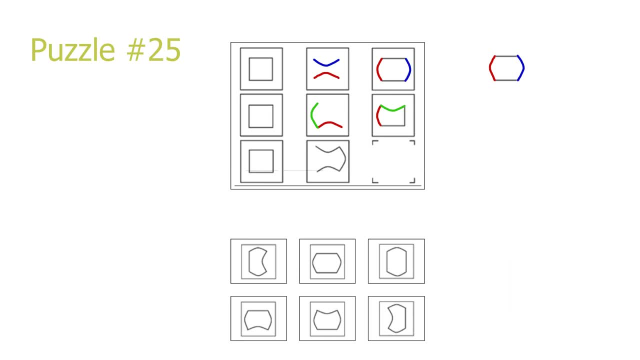 in the row and finally, we remove the extra line which is inside our shape. This gives the third picture in the first row. So, yeah, the second picture in the row always describes the inverse curvature, 90 degrees in clockwise direction, which will happen in the third picture. 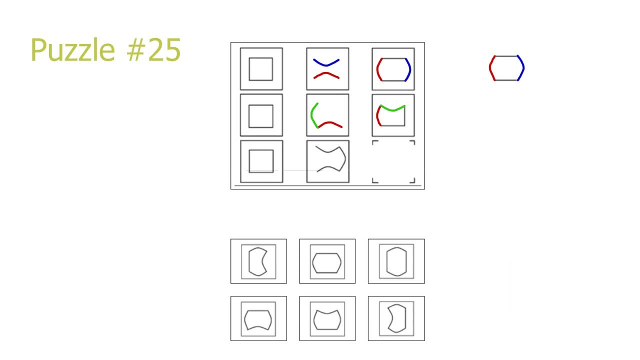 To solve the puzzle, let's look at the last row. The second picture has two inward curved lines on the top and on the bottom. This corresponds to two outward curved lines on the left and on the right. in our answer, This leaves 2,, 4 or 5 as the correct answer. 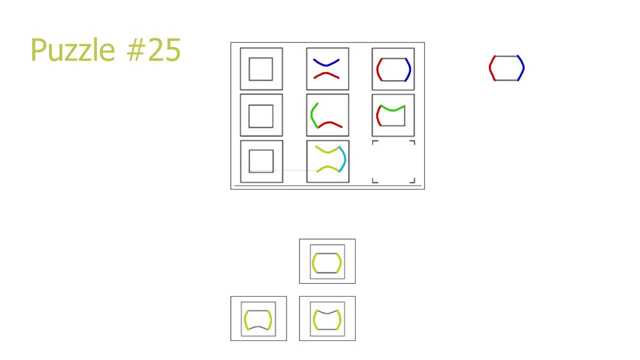 Puzzle 27.. We have this outward curved shape on the right side. Inverting the curvature and rotating it 90 degrees leads to an inward curve. on the bottom side of our answer We can see that answer 4 has both this outward curvature on the left and right side and inward. 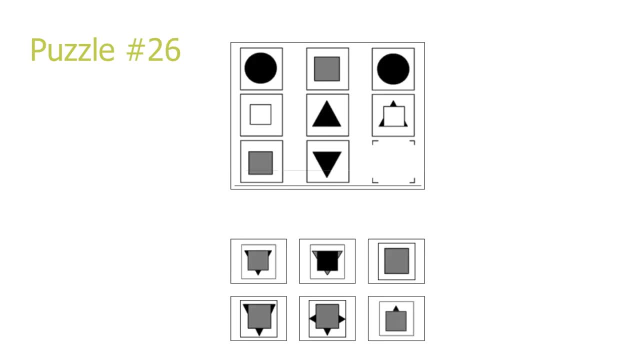 curvature on the bottom side. 4 is the correct solution. Puzzle number 26.. Before I solve this puzzle, I would just like to mention that solving this puzzle requires a good eyesight, so in my opinion, this puzzle should never be on an IQ test. 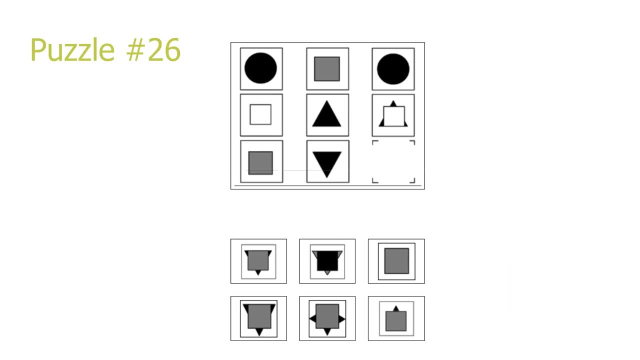 But yeah, let's solve the puzzle. First of all, this is a row puzzle. Looking at a specific row, we could see that the third picture is just the first picture in front of the second picture. To solve the puzzle, we just look at the third row and we get that. our answer is a grey square. 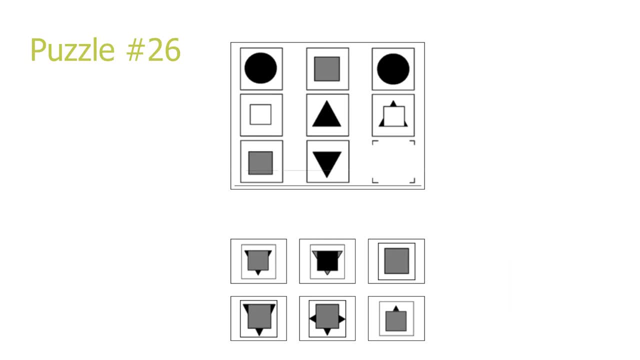 in front of an upside down black triangle. Before I tell you the problem with this test, let's just eliminate the obvious incorrect answers. Answer 2 cannot be correct because it has a black square. Answer 5 cannot be correct because it has a black star shape instead of our black triangle. 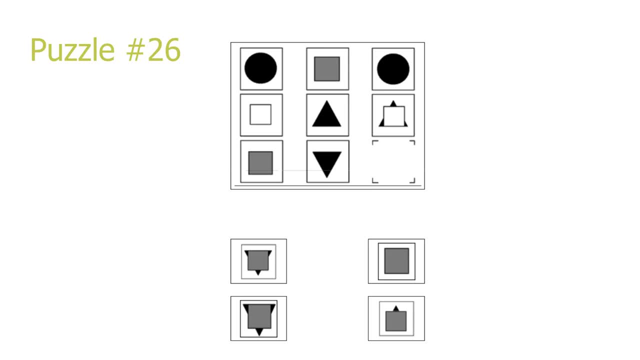 And answer 6 cannot be correct because it has a triangle pointing up. Answer 7 cannot be correct because it has a black star shape instead of our black triangle. And answer 8 cannot be correct because it has a triangle pointing upwards while our triangle is pointing downwards. 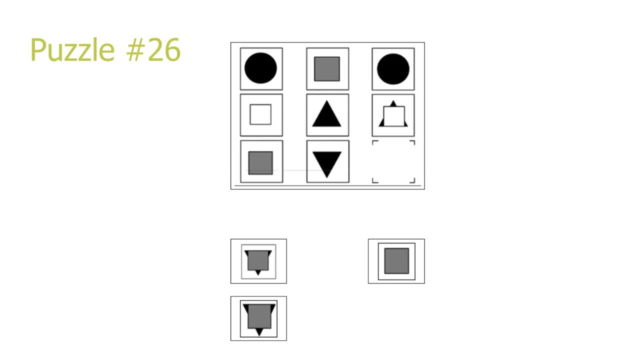 This leaves these three answers. My problem here with this puzzle is that how are we supposed to determine which one is correct? Answer 1 can be correct because it has a black upside down triangle behind a grey square. Answer 3 can be correct because if we look at our square in the third row and compare. 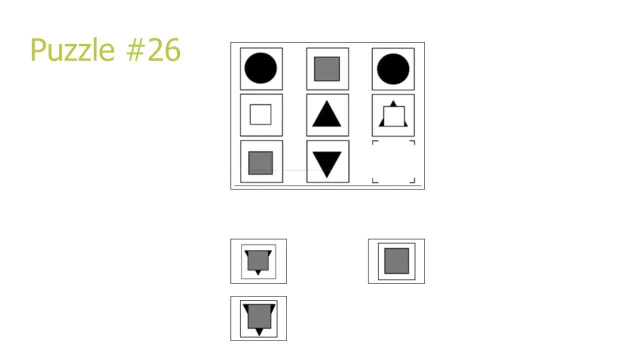 it to the square in the second row, we can see that our square in the third row is actually bigger than the square in the second row, So the grey square might be big enough to hide the triangle completely. And answer 4 is pretty much identical to answer 1, so it can be correct as well. 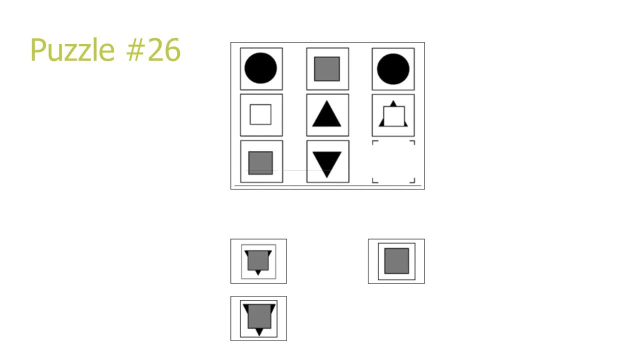 It is actually possible to determine which answer is correct, but it requires a good eyesight. First let's see why answer 3 is not correct. If we look at the third row and compare the height of the triangle with the height of the square, we can clearly see that the triangle is a bit taller than the square. 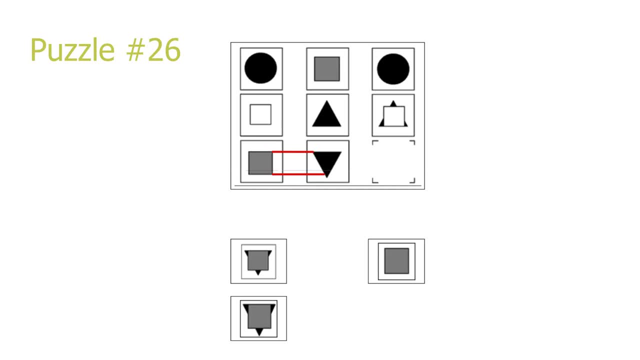 Therefore the triangle would either stick out on top or bottom of the square. So answer 3 is not correct. Now let's see why answer 4 is not correct. Answer 3 is not correct. Answer 3 is not correct. Answer 3 is not correct. 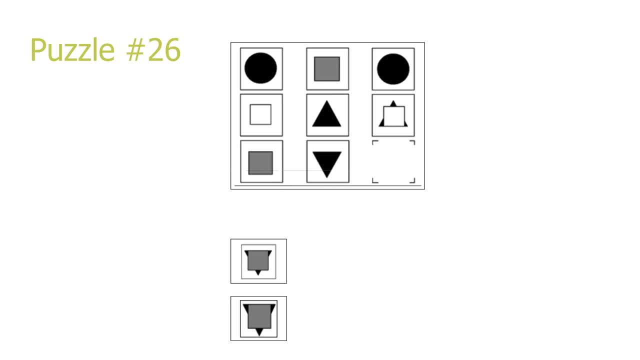 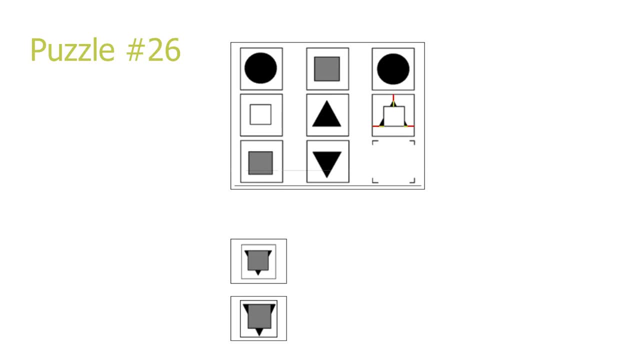 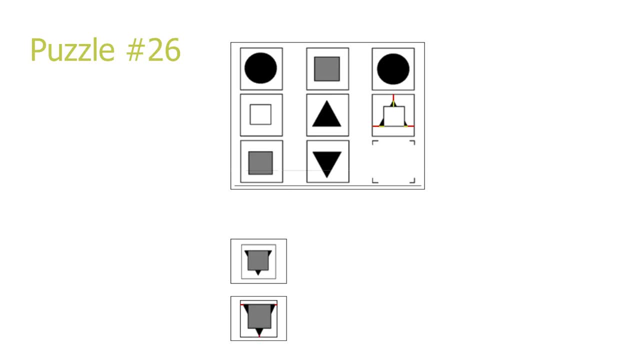 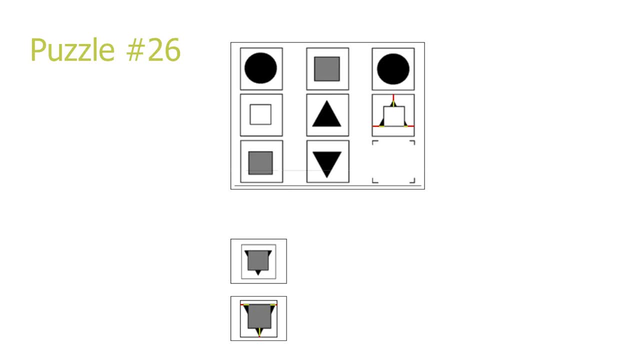 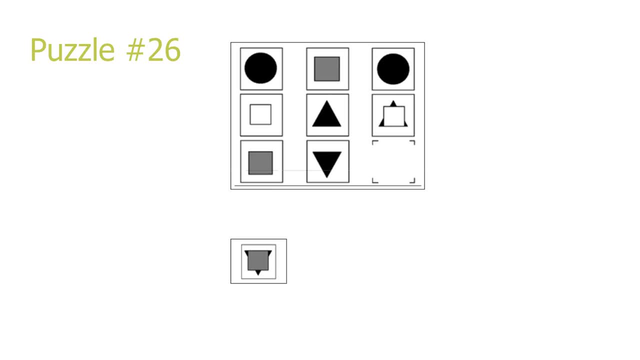 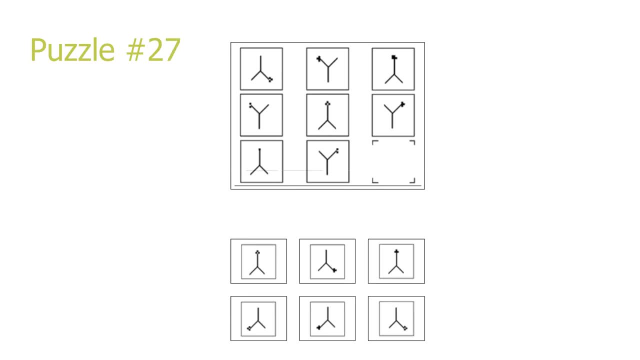 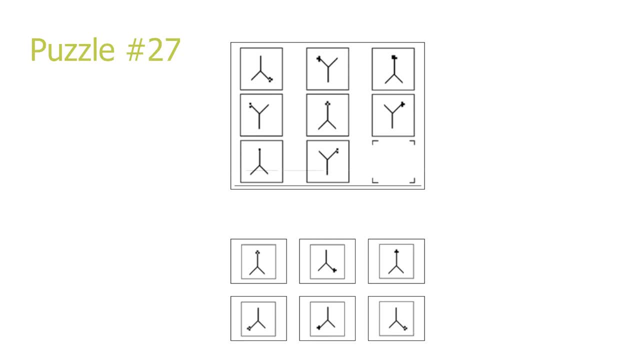 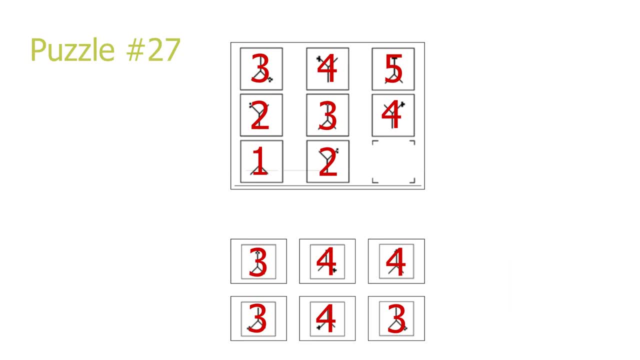 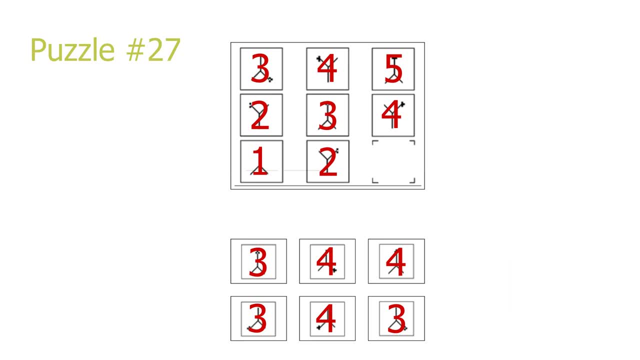 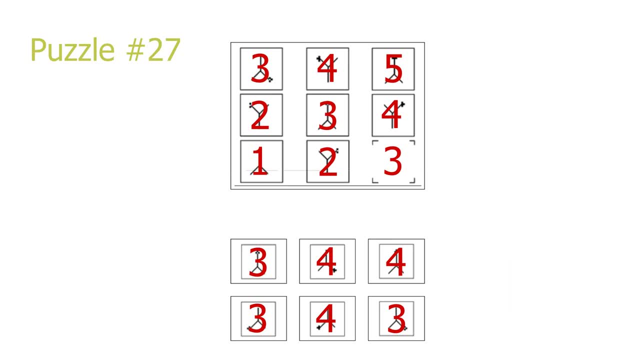 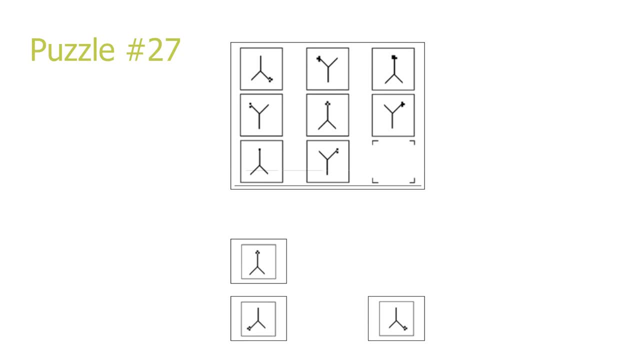 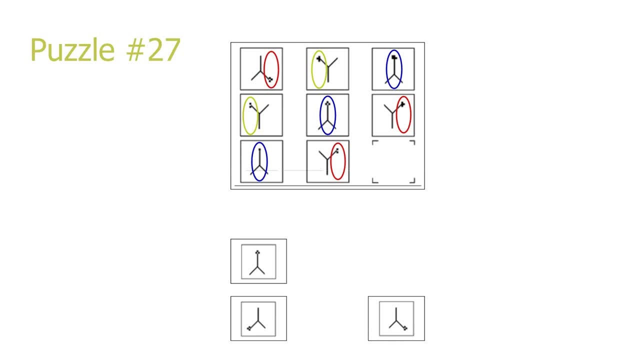 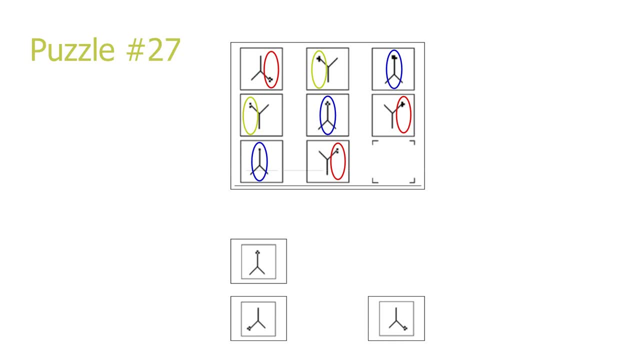 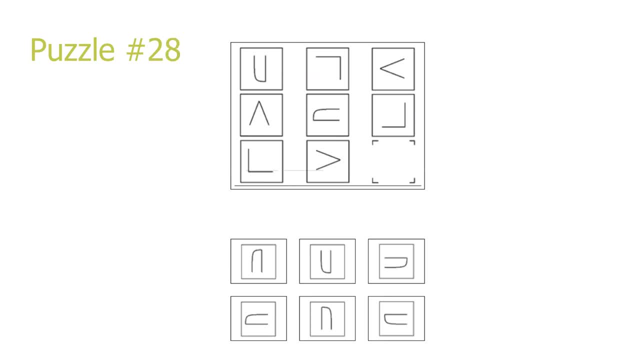 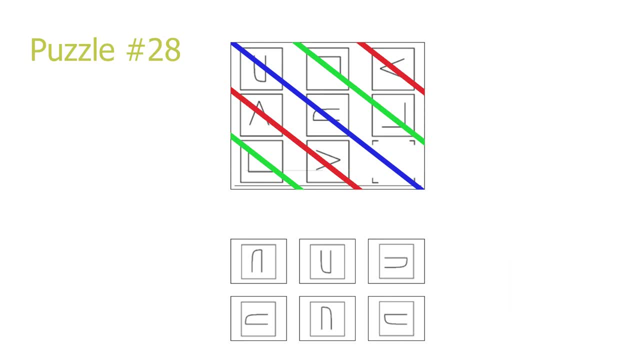 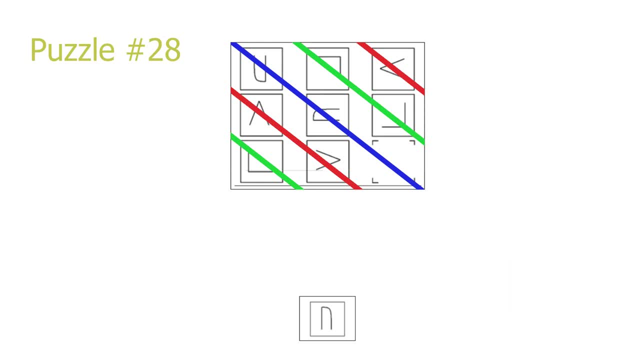 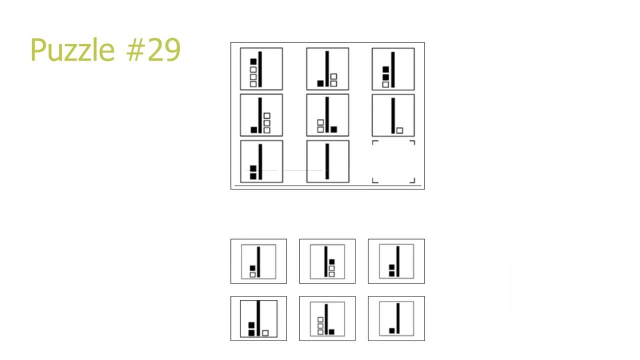 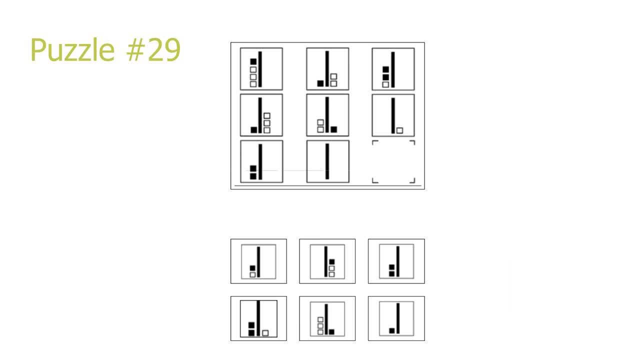 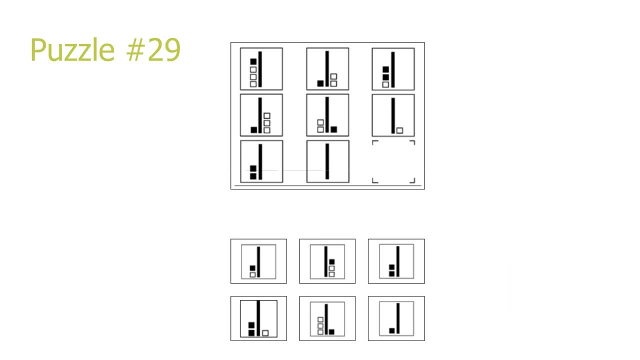 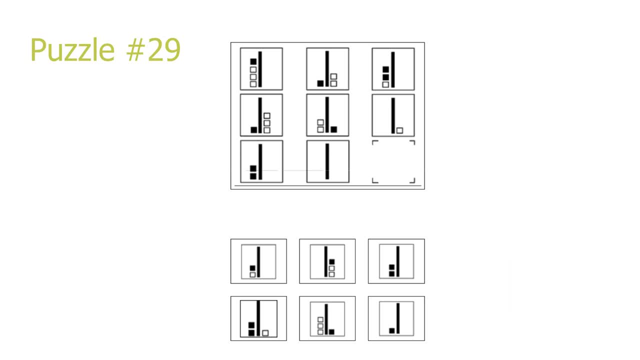 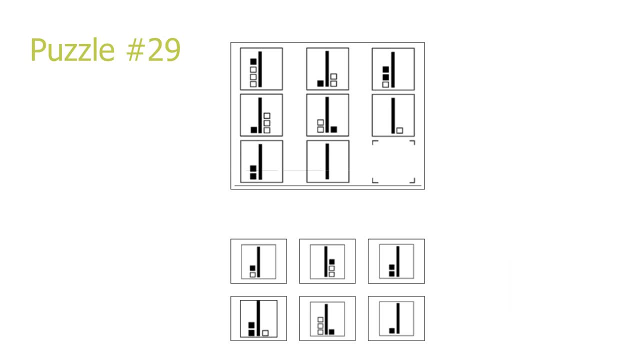 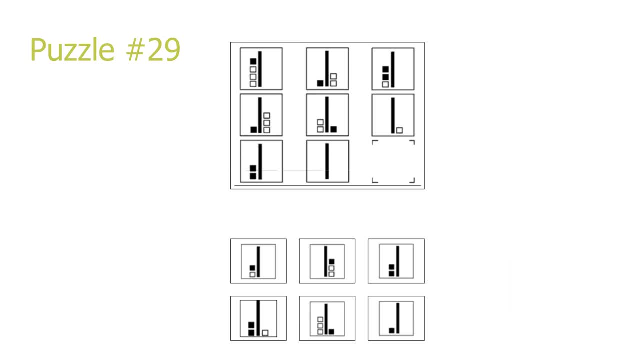 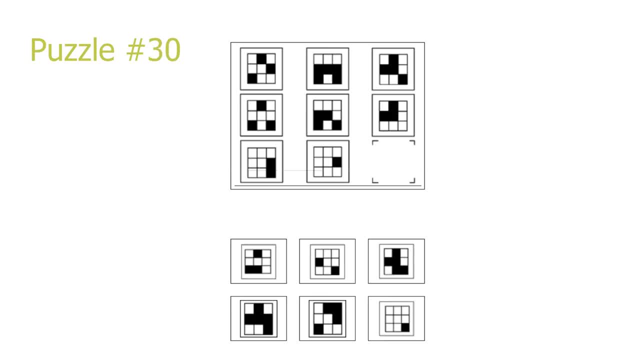 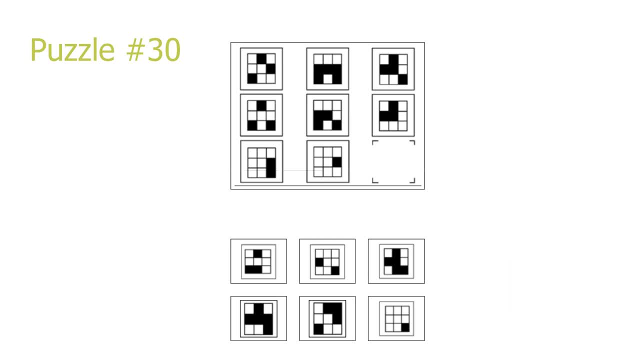 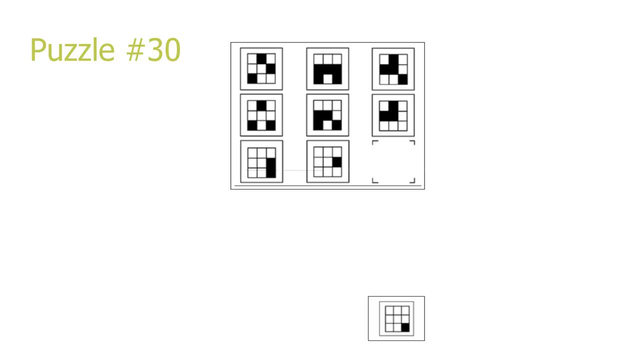 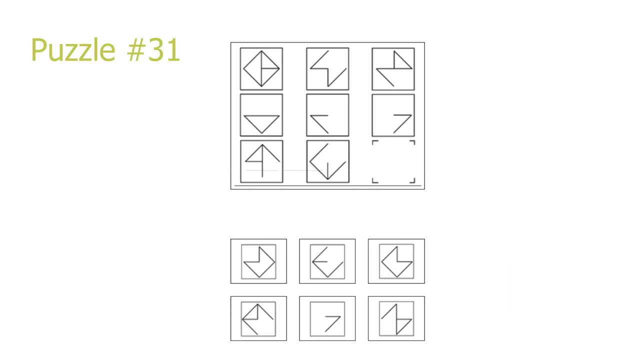 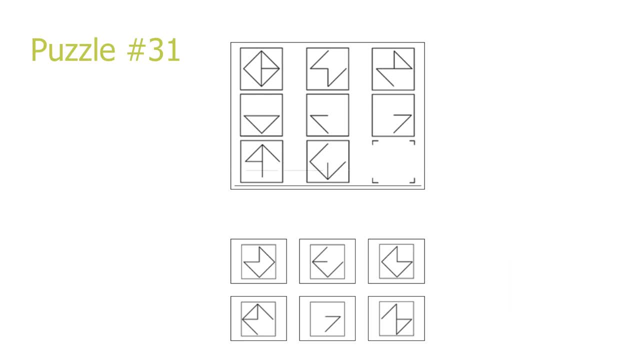 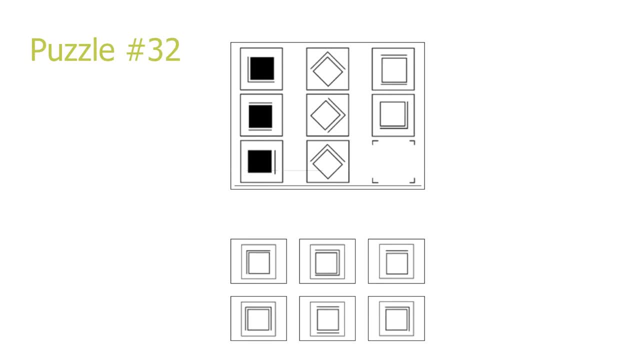 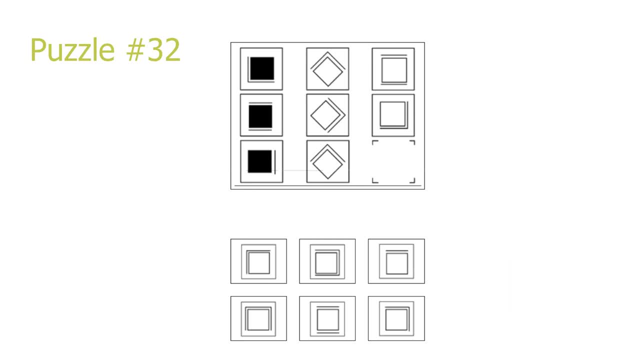 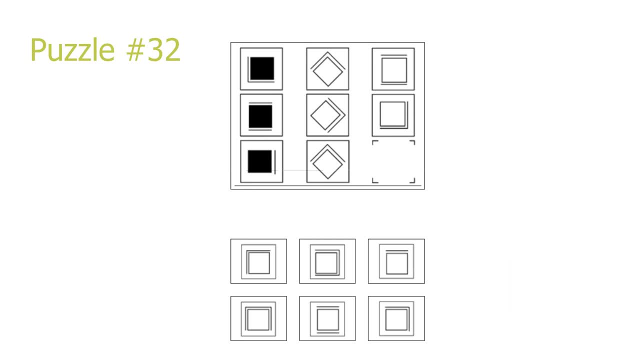 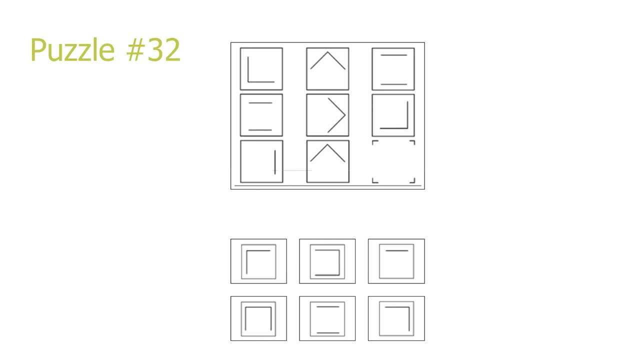 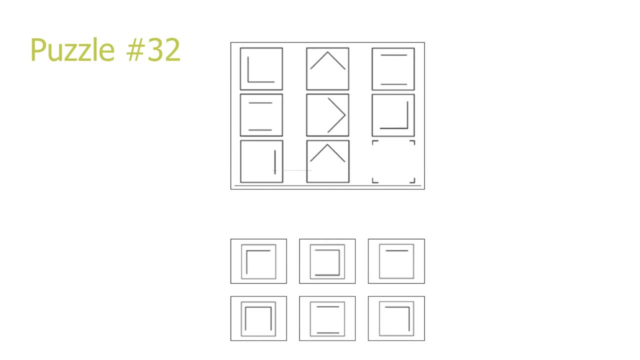 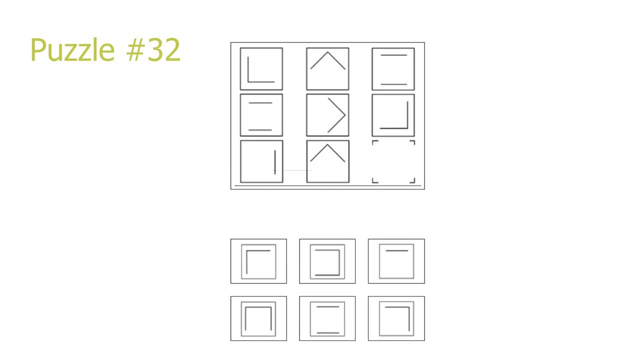 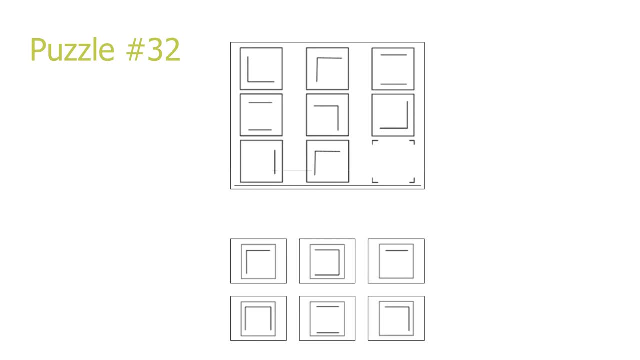 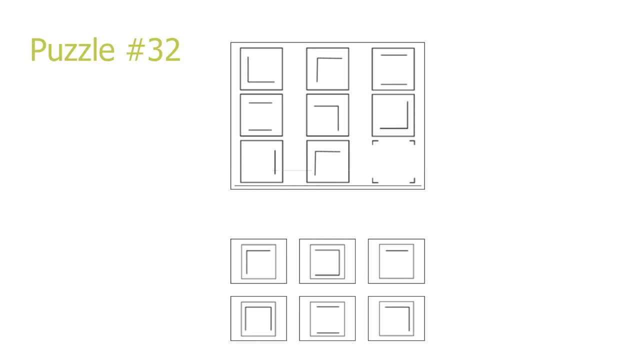 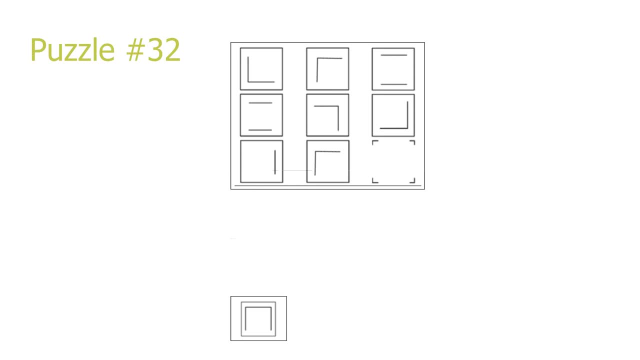 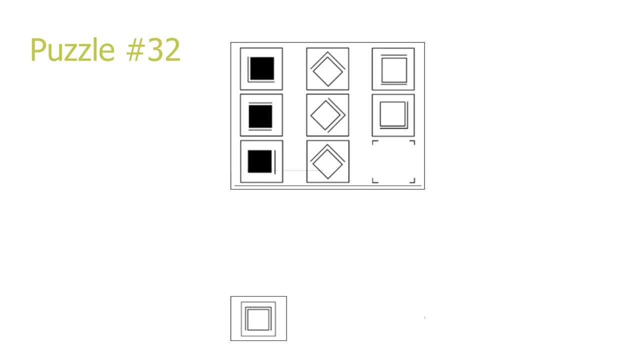 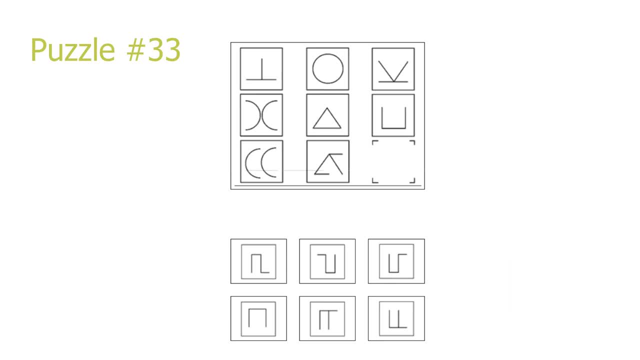 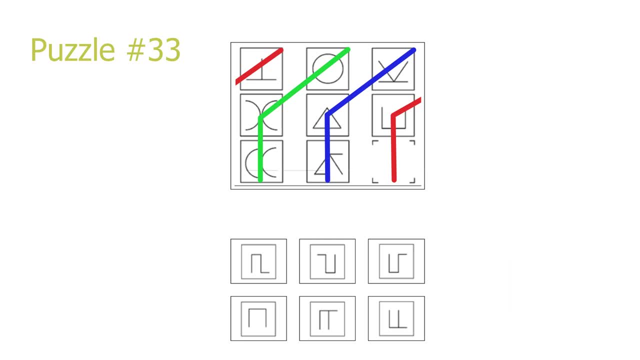 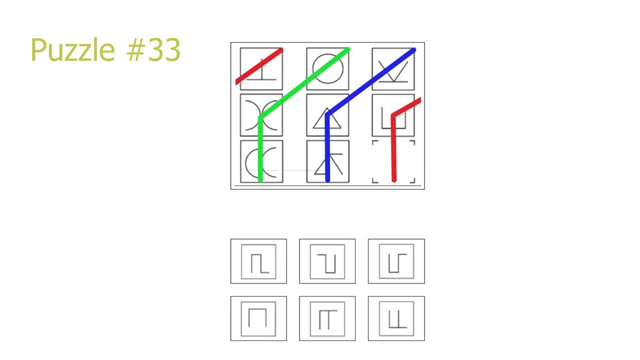 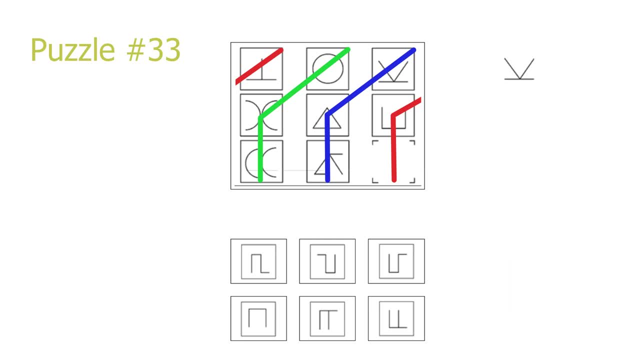 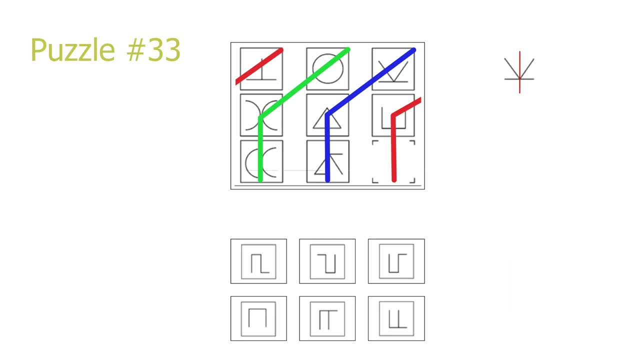 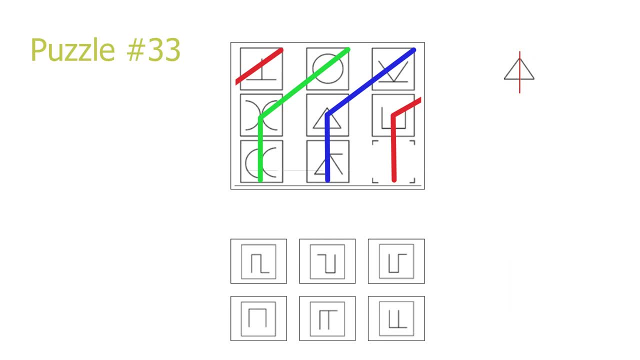 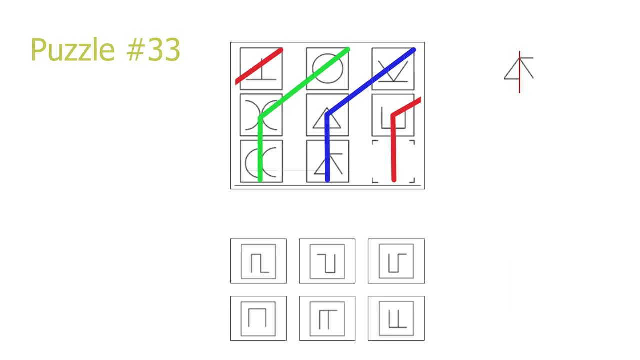 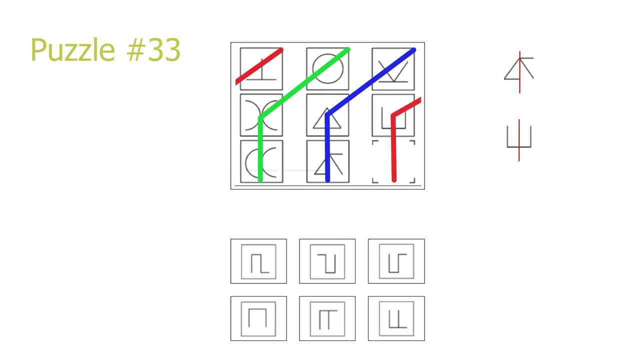 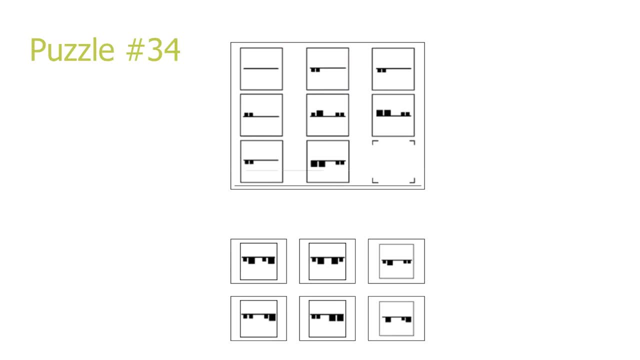 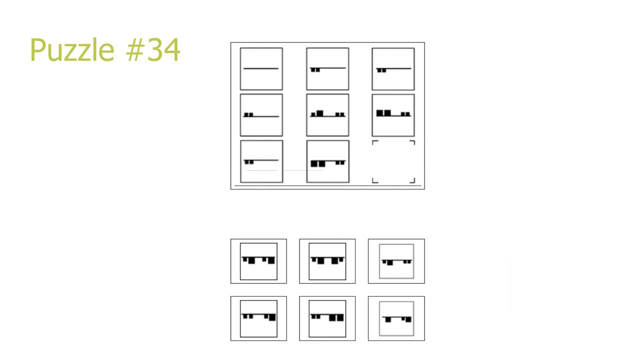 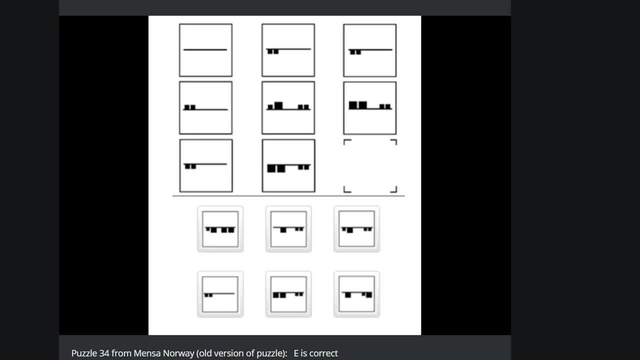 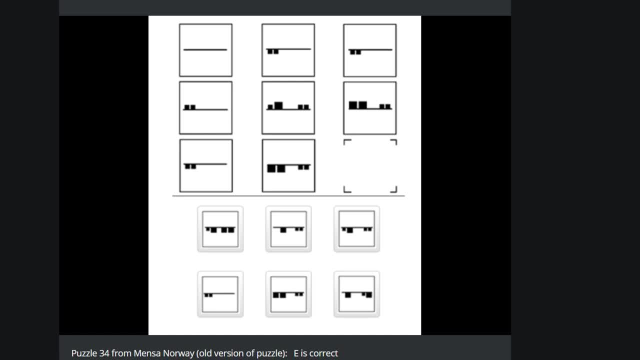 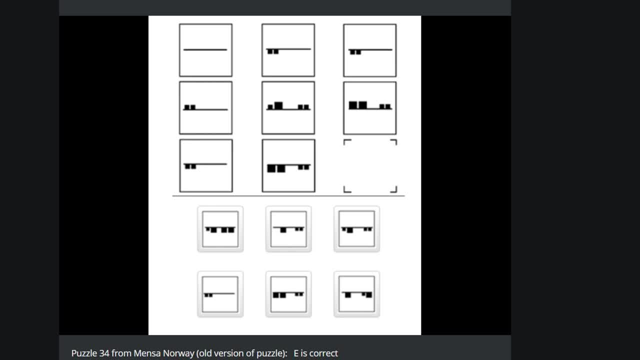 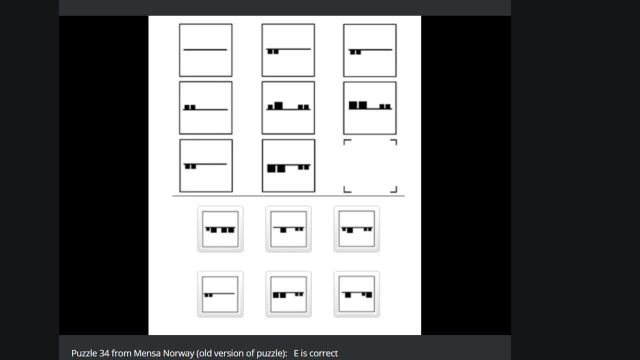 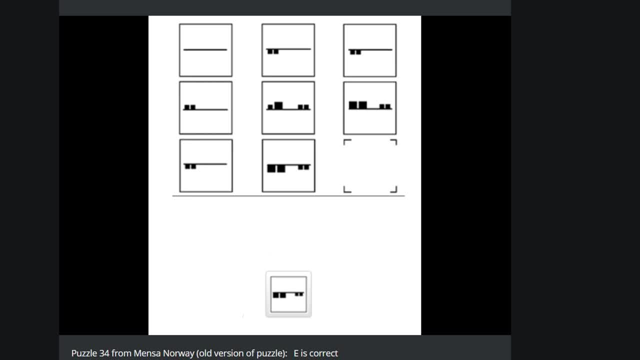 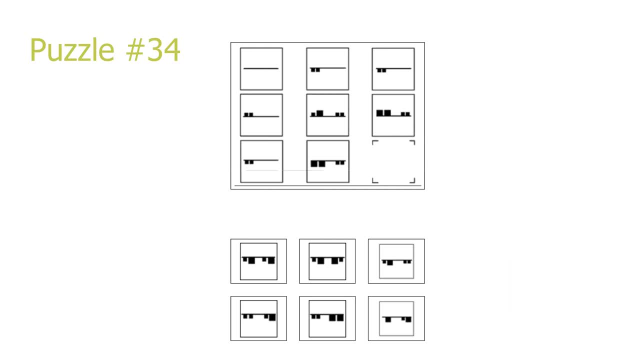 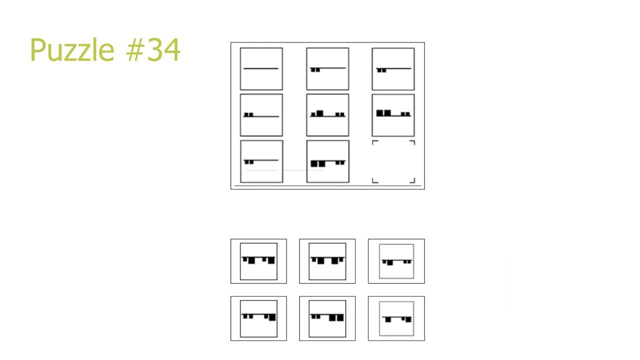 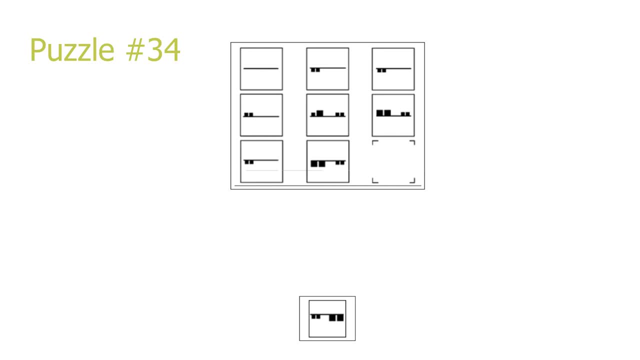 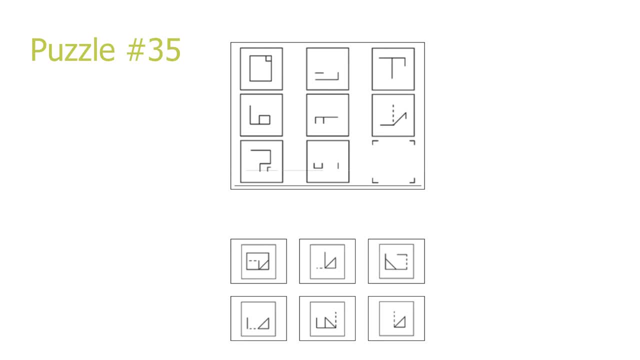 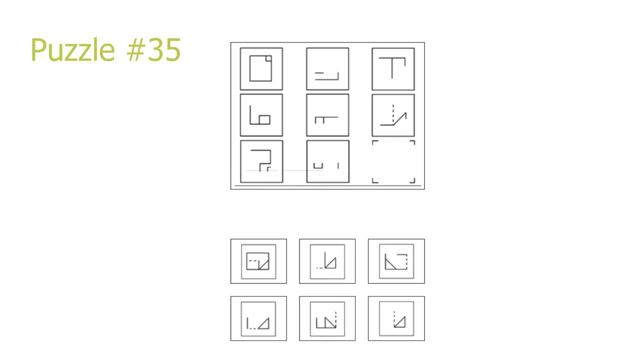 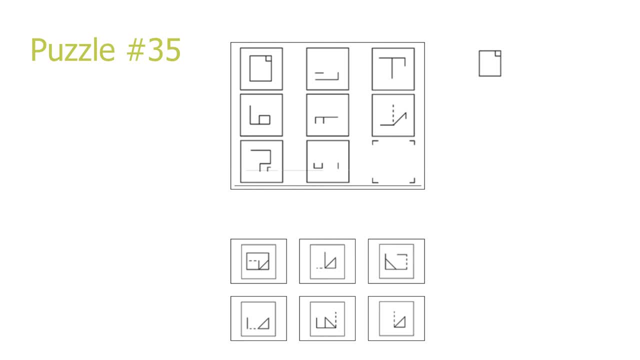 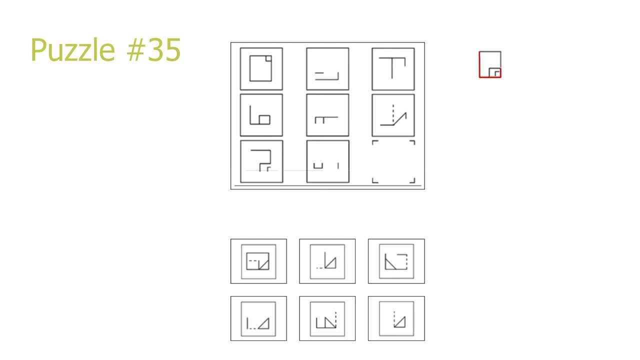 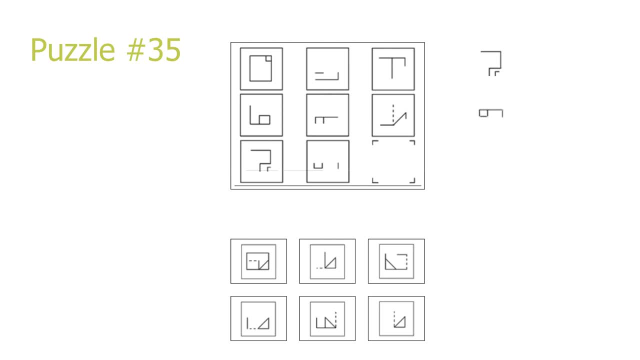 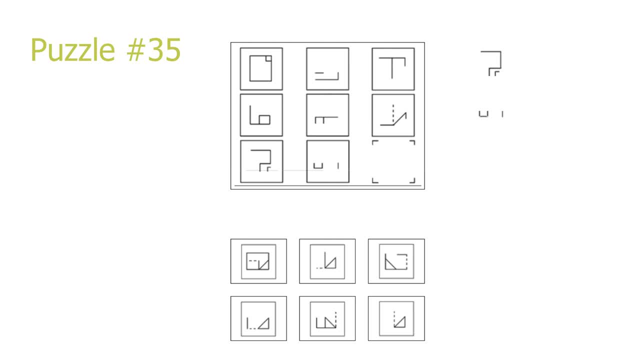 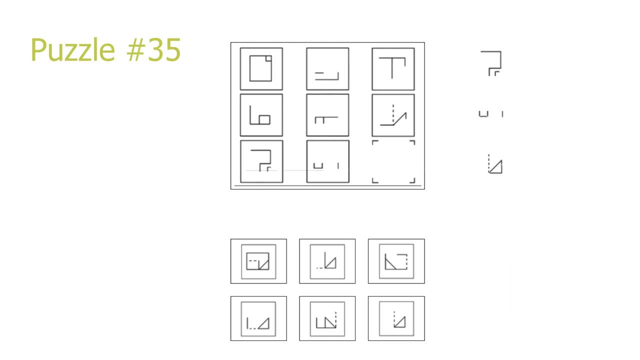 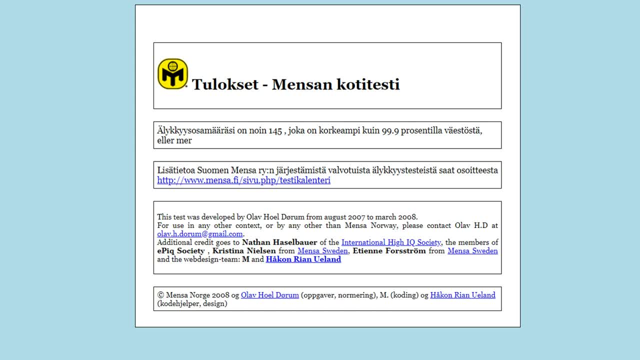 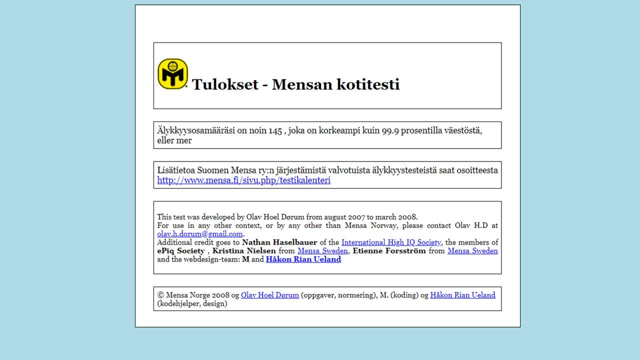